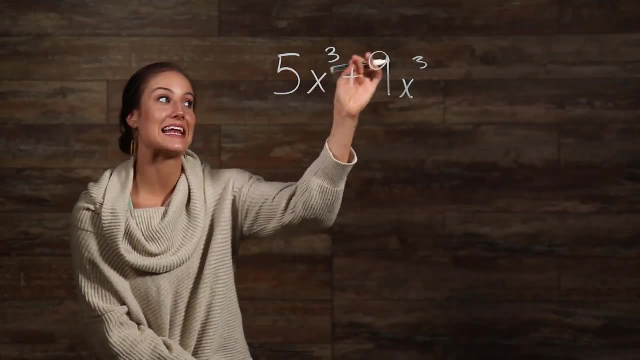 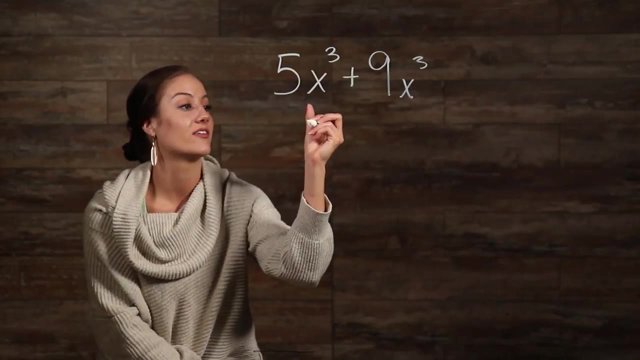 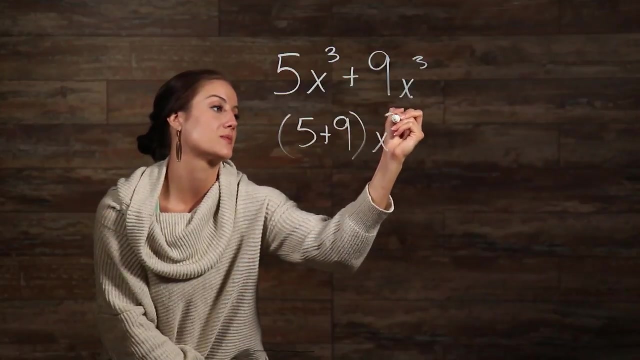 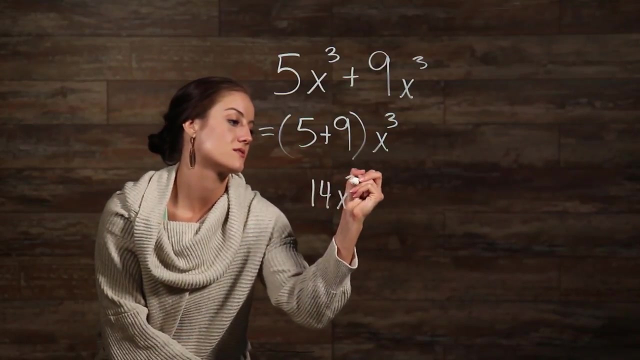 Add the coefficients together, but leave your base and exponents the exact same. In this problem, our coefficients are 5 and 9.. And 5 plus 9,, so we're leaving our base and exponent the same. So, leaving our base and exponents alone, we get 14x to the third. 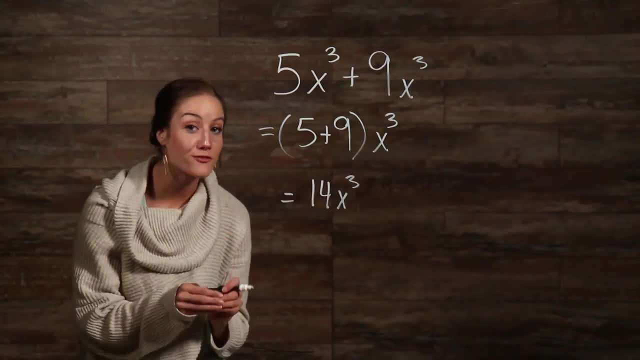 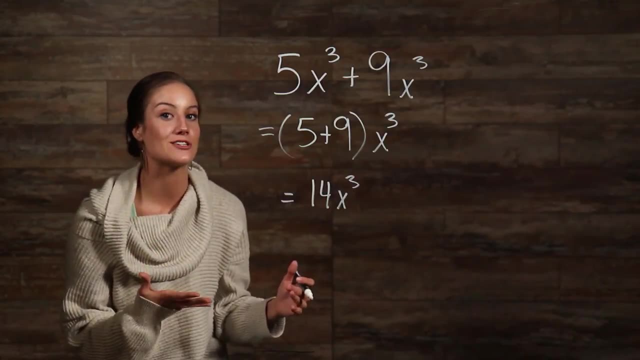 Remember to add or subtract numbers that have exponents. you must first make sure that the base and exponent of the two terms you're trying to add or subtract are the same. If they are the same, then all you have to do is add together the coefficients and keep the base and exponent the same. 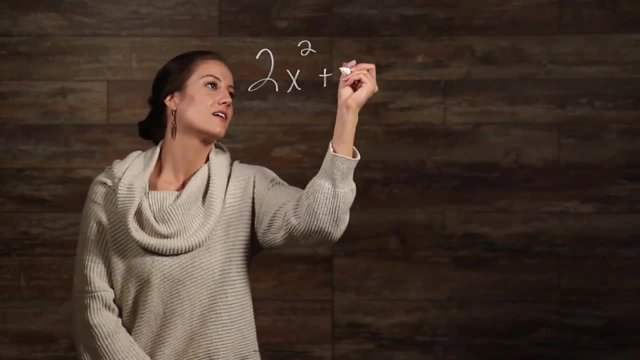 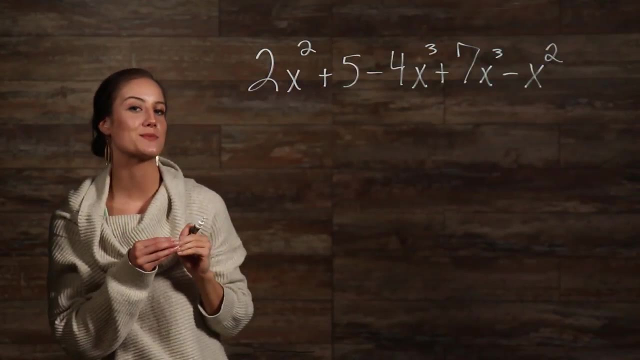 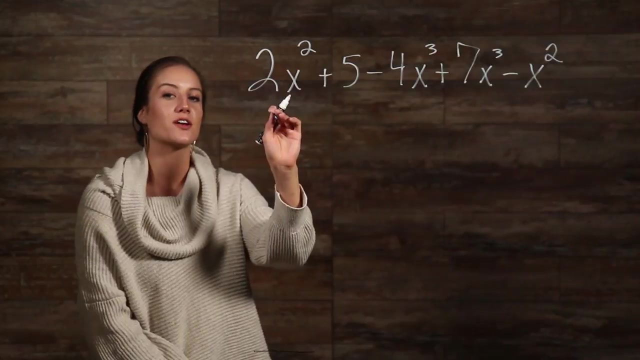 Let's take a look at another example. Alright, so in this example, some of the terms have different exponents, so we need to identify all of our terms that can be combined together in order to simplify this expression, Starting with our 2x squared. are there any other terms with an identical base and exponent? 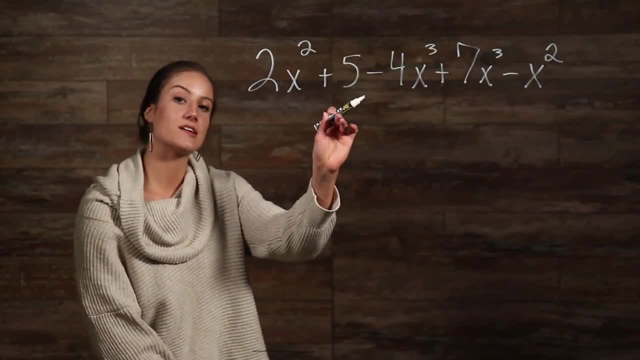 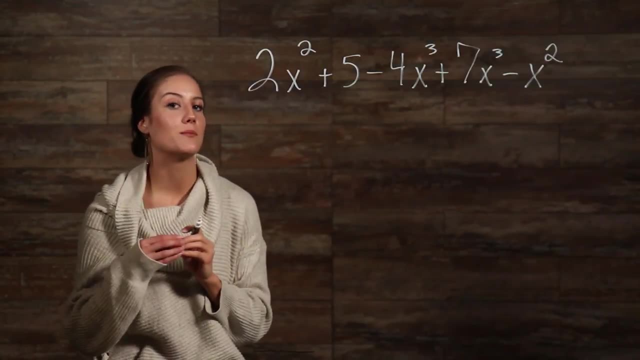 Yes, Our negative x squared, our 5 is on its own and negative 4x cubed plus 7x cubed share identical base and exponents. We know that to combine our like terms together, all we need to do is add together the coefficients of the corresponding like terms. 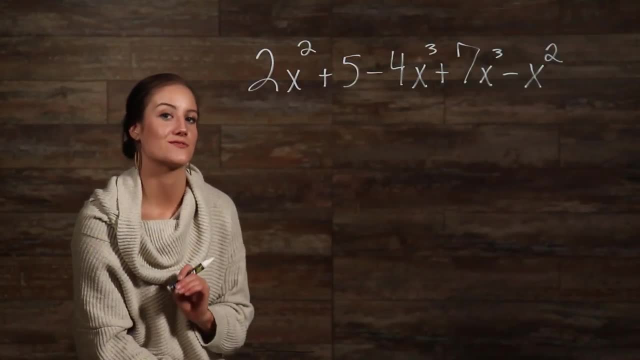 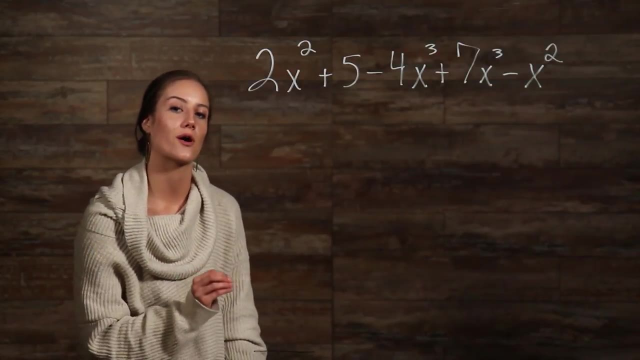 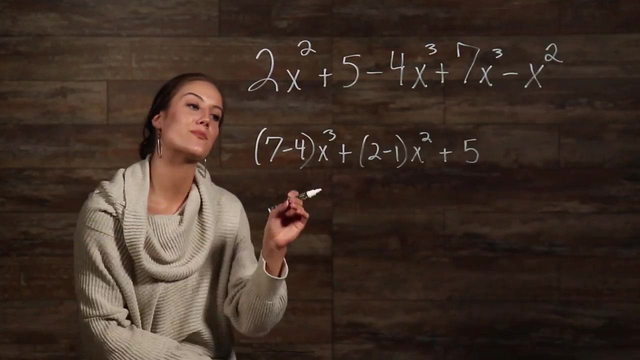 So here's how we can do that. Since we're adding together the coefficients of 2x squared and negative x squared together and all other like terms, we can rewrite this expression to help us follow our work. Now, the reason that I brought my term with a 3 in the exponent to the front is because in the standard form of a polynomial equation, 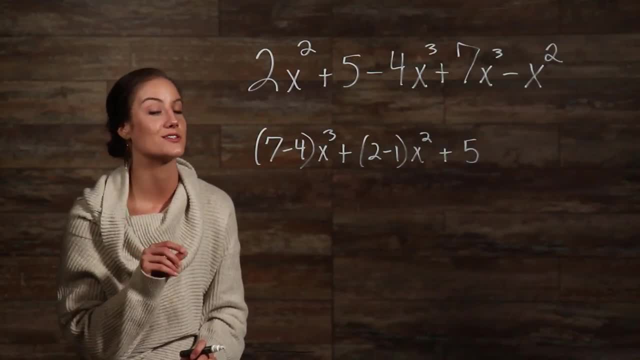 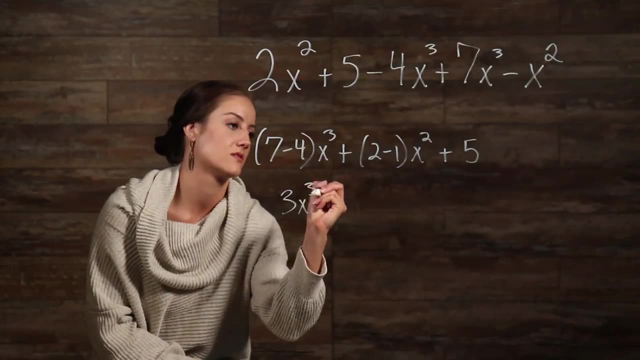 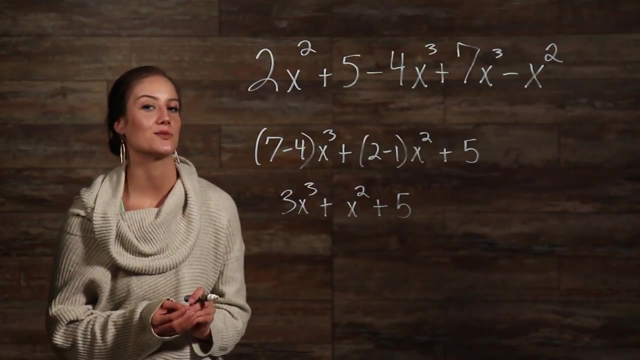 you always bring your term with the highest number in the exponent to the front or to the left. Now, when we add our coefficients together, we get At this point: all of our terms have been combined and there's no further simplification that we can do. 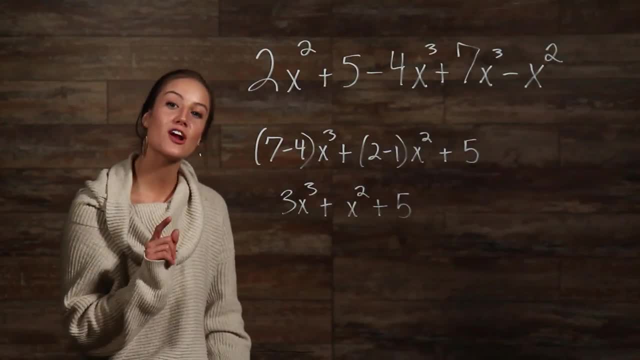 So we're done. I hope that this video was helpful And, for further help, be sure to check out more of our videos by subscribing to our channel below. See you next time.